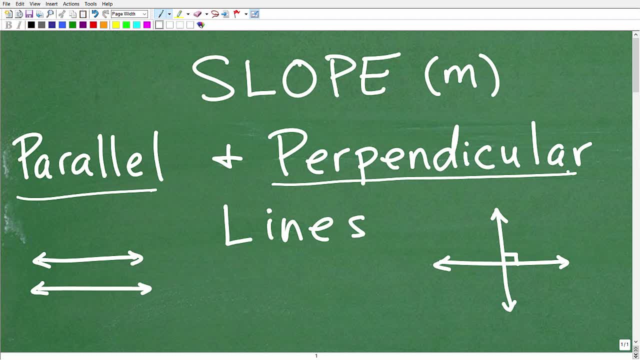 Tablet Class Math. I'm also a middle and high school math teacher And over the last several years I've constructed many online math courses, mostly in the middle and high school math courses. I've also done a lot of math courses in the middle and high school math courses. 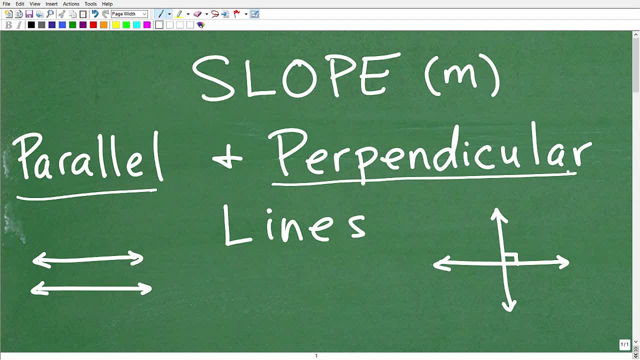 So I'm going to leave a link to my full learning program in the description of this video. So this is like a tutorial video, But if you want my complete full instruction on all math topics, then you definitely want to check out my math learning program. Also, if you're new to my 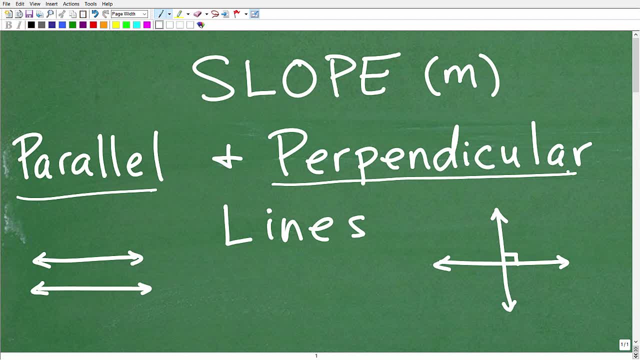 YouTube channel. hopefully you consider subscribing. I already have hundreds of videos on my YouTube channel. I can help you out in math and I'm posting stuff all the time, And if you find this video helpful, please smash that like button. So without further ado. 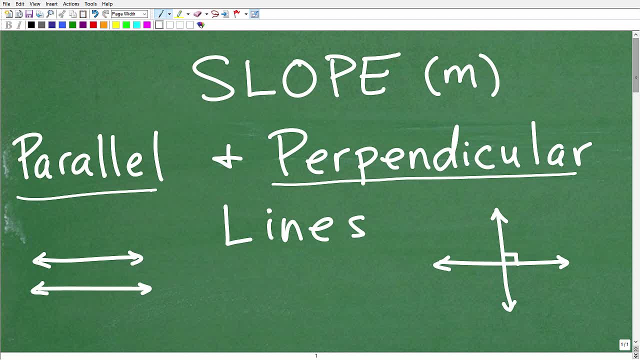 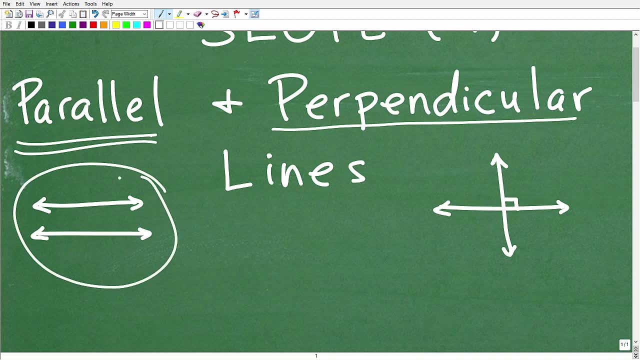 let's go ahead and get to the topic. All right, So here, parallel right These two lines are, you know, basically are parallel right. They, you know, not perfectly parallel, because this is a sketch, but this is the idea of parallel right, One line next to another line, And these two lines, 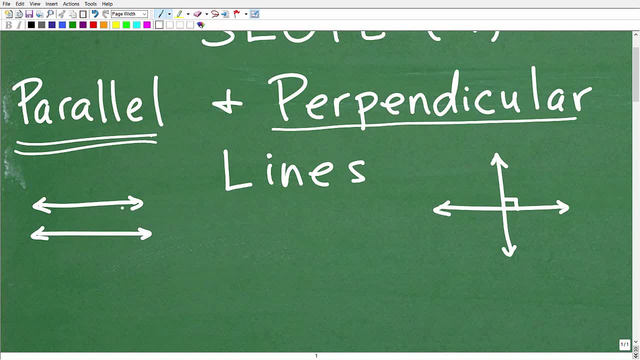 will never cross, right, They're never going to intercept because they're just side by side, parallel, kind of like railroad tracks, if you will right, They're never going to cross. So when you see a line like this and another line, 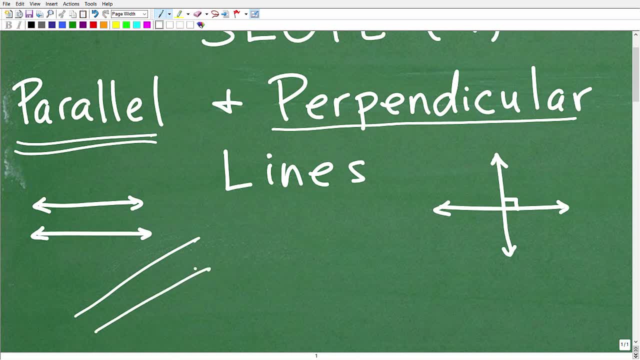 next to it. those lines are parallel. Now, perpendicular has a very specific definition, And that is where a line is. They're obviously crossing, but they're crossing at right angles. Okay, So, 90 degrees, All right. So it's not just that they're just crossing like any old way. 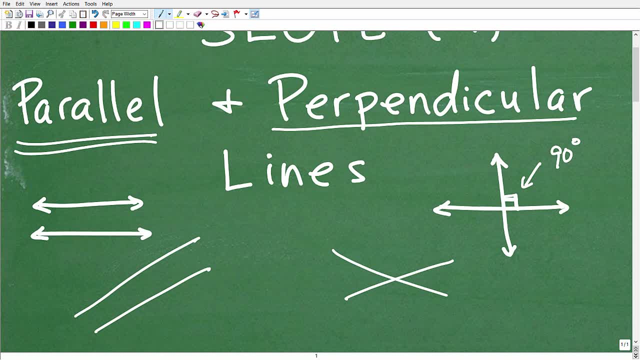 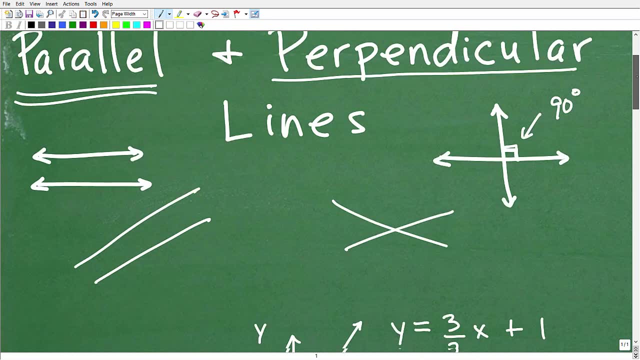 They're specifically crossing at 90 degrees. So lines that are like this are perpendicular and lines that are like this are parallel. Okay, So let's get to a problem here, And we're just going to focus on this one problem, because, again, 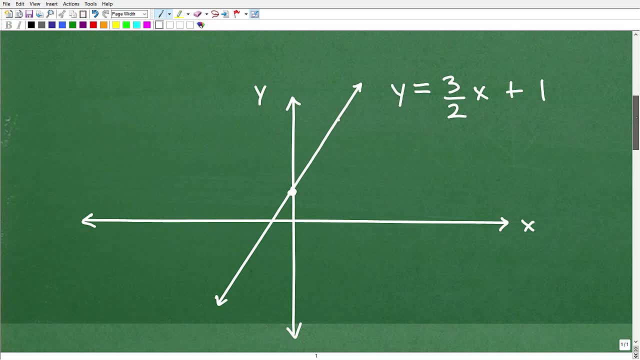 there's a lot of sub skills that you need to be good at to handle problems that involve the equation of lines that are parallel to one another, perpendicular, et cetera. So let's just talk about a few of those Again. check out my more of my videos on my YouTube channel, If you. 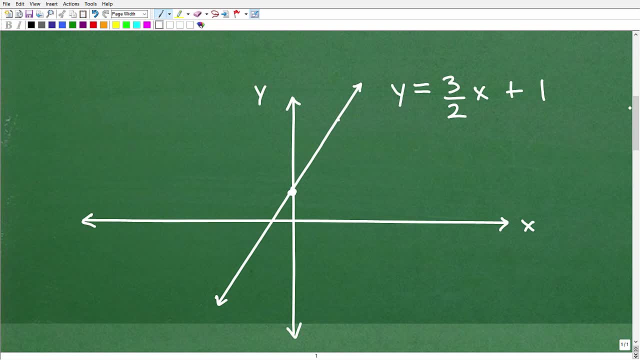 want to kind of learn about that. I guess the best almost organized way to learn that is to go into one of my math learning programs. So I'm going to go into one of my math learning programs, But you know, let me just focus here. Right? So here we have an equation. Okay, What type of 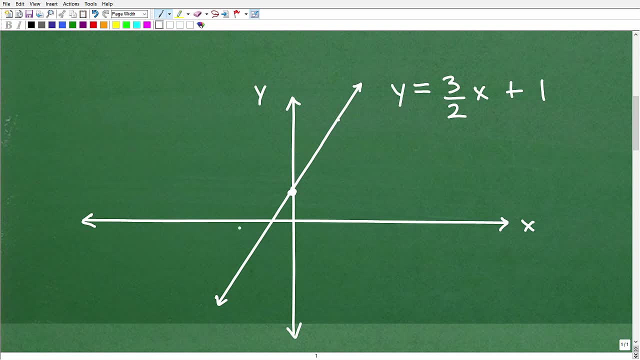 equation is this? Well, it's. this equation represents this line. We call this a linear equation, Right? So this is a linear equation and it's a algebraic representation of this line. Okay, So this is a line and this is this line's equation, or a linear equation. Okay Now. 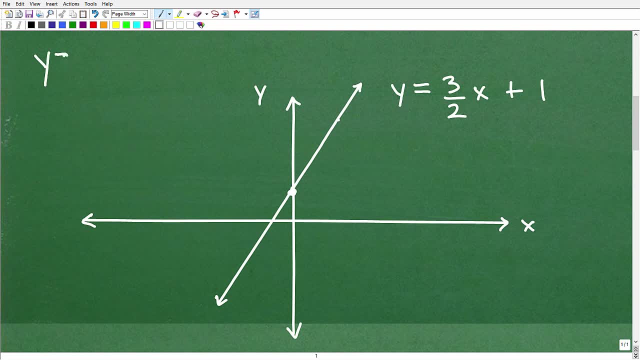 hopefully you knew that. Now, one of the most common ways to write the equation of a line is this way: y equals mx plus b. Okay, So you could see this. y is by itself. Okay, So here there's y. Then we have an equal sign, just like: 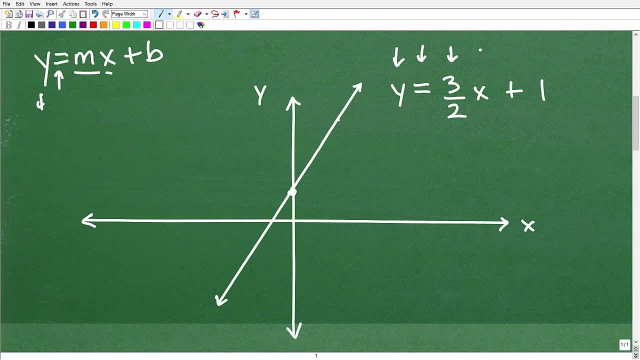 that. And then we have an m and x, So m and x, So this m. okay, that's a particular value In this case. in this example, the m is three halves three over two, And then I have an x plus a, b. 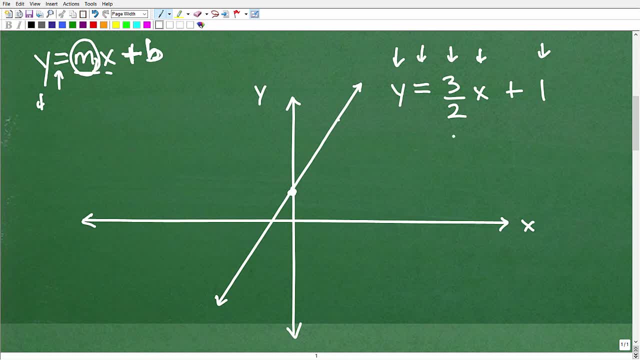 That's just some other value. In this case it's one Okay. So here m is three halves and b is one Okay. But the main thing I want you to know is that this line okay, this example right here: 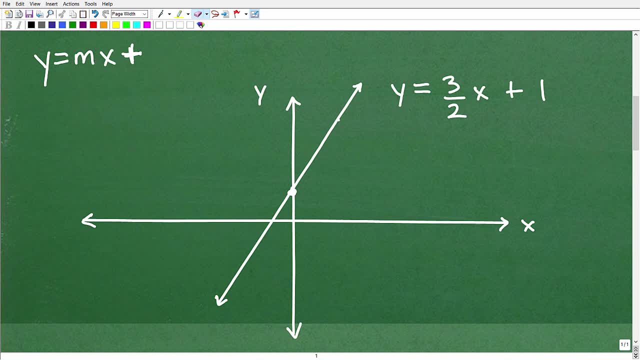 right is: in this format, y equals mx plus b. Okay, So the convenient thing about this is that we can graph. lines are in this format. This is what we call the linear equation. Okay, So this is the slope intercept, y intercept form. Okay, Now I don't want to take this video down the path. 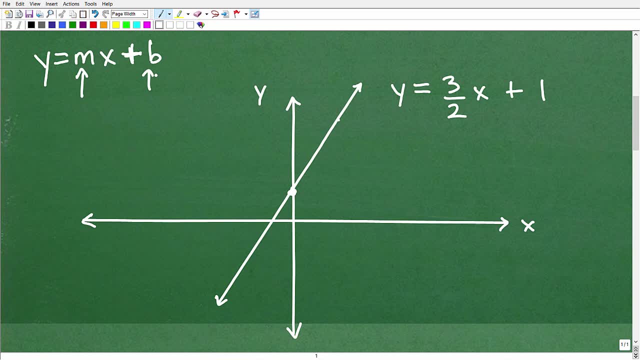 of how to graph lines, Okay, But I do need to kind of review some of this stuff with you just to make sure that you know you're not going to be confused about anything, Right? So that's, this is the kind of what I'm doing. I'm just kind of setting you up here, Right? So now, 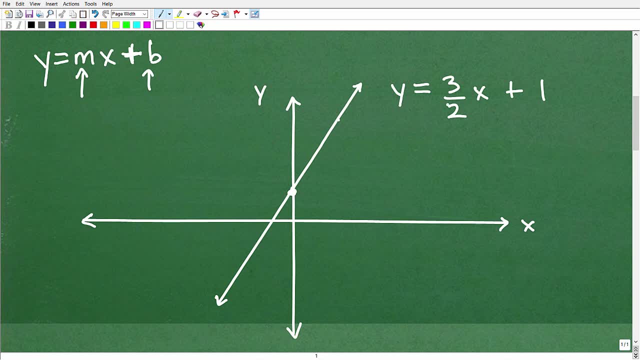 again, here is this line, Here's the equation of this line. The slope is three halves. Okay, That is the slope, All right. Now the slope is the rise over the run. Again, there's a lot to know about the slope, Okay, But basically the main concept about the slope that you need to know. 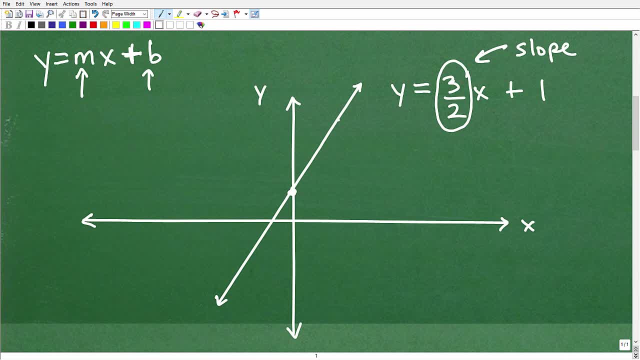 is that the slope is a, is a number, is a value that expresses the angle of this line. Okay, So each line, depending on what its angle is, is going to have a different slope to it. Okay, So that's kind of the big picture. So if we have a line that is, 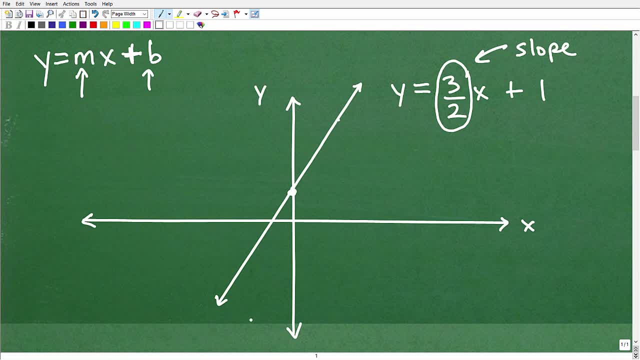 is parallel to this line. let me just kind of sketch one like: so All right, This line here, this has a slope of three halves. Okay, It's, it's steepness or its angle is three halves. So lines that are parallel to one another have the same slope. That's just all you need to know. 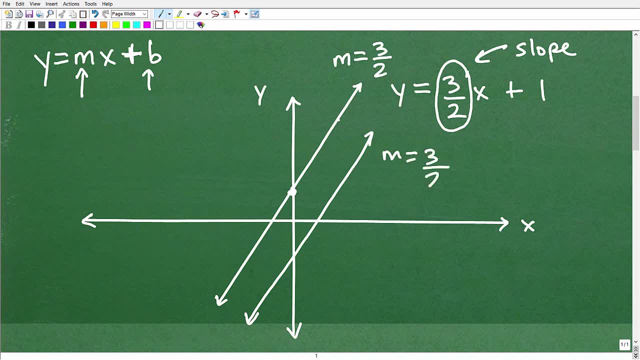 So this line down here has a slope of three halves as well. It's as simple as that. So two lines that are parallel one to one another have the same slope. Now remember this one. okay, had to do with this. this plus B, this Y intercept, Okay, So in other words, our first. 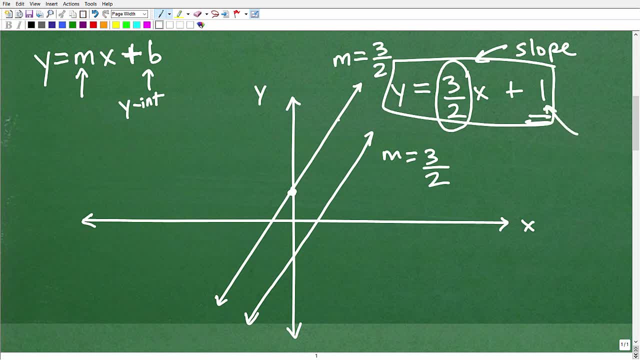 line right here. the one is a representation of where this line chops through the Y axis. So that would be like a one. Okay, So this line with the slope of three halves crosses through or intercepts the Y axis at one. Okay, So let's just kind of make up a another equation of this line down here. Okay, Now this: 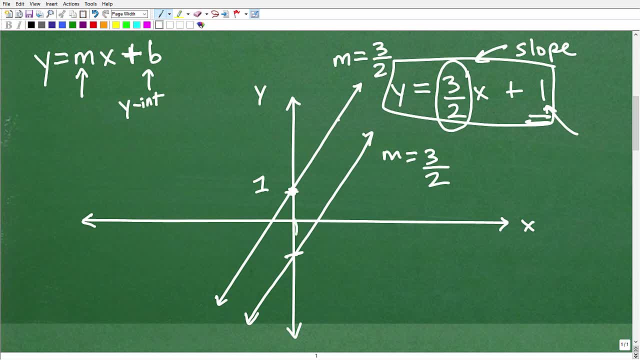 is a little bit further down. So what would, could possibly, what would be a reasonable guess at this line right here, an equation of this line, right? So maybe, like Y equals what? Well, it has to have the same slope, because these are kind of, these are parallel to one another. 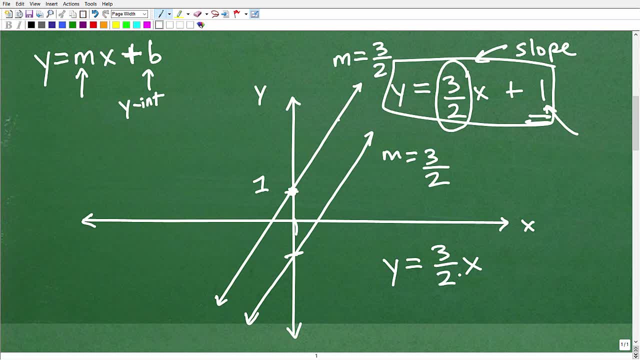 So we're going to have to put three halves X, but they're going to have a different Y intercept, So this might be intercepting, at, say, negative two. So I would put minus two, Okay. So when you're looking at two lines, let me go ahead and just erase this, If I was to ask you. 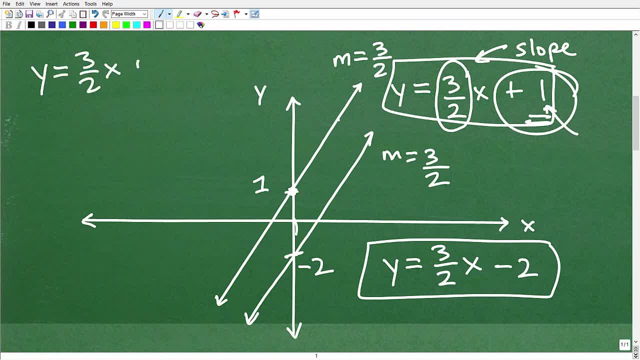 are the lines Y equals three halves X plus one and the lines Y equals three halves X minus two. are these lines parallel to one another, or perpendicular to one another, or whatever? Okay, Oh, they're both. in. Y equals MX plus B form. Okay, They have the same slope, Okay So. 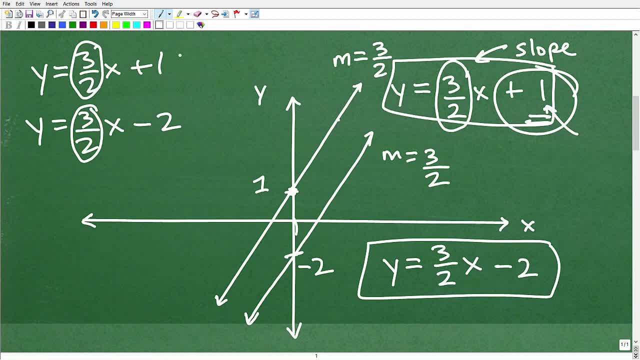 they're definitely going to be parallel, Okay, And here they're not the same line because they have different Y intercepts. Okay, All right. So that's a quick overview on two lines that are parallel. Just remember, two lines that are parallel to one another are going to have the. 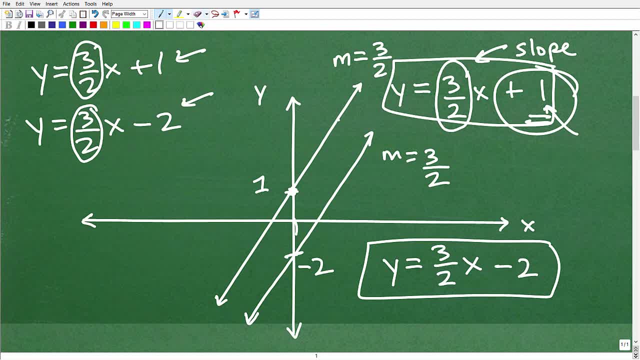 exact same slope. That's the main thing you need to be comparing them to, but you have to have the lines in the same format. okay, it's not going to do any good to have a line like, say, 3x plus 4y equals 12 and y equals two-thirds x minus five. right? so to do this comparison, to know whether 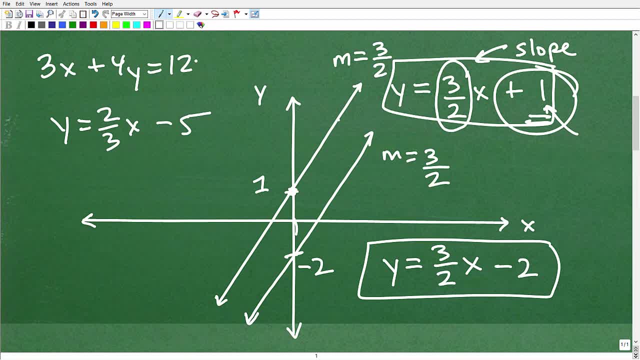 these two lines are parallel to another. you're going to have to go ahead and rewrite this- this guy, right here in terms of y. okay, then that way you can kind of see it like: so again, a lot of sub skills going on here, but the main idea is this: you're focusing on comparing the slope. you. 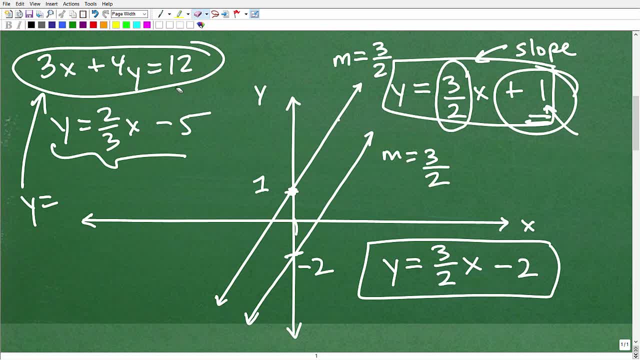 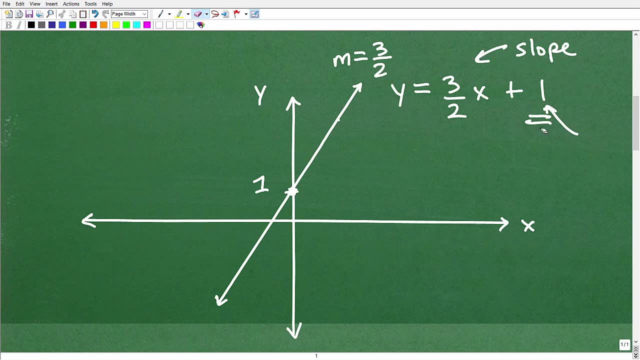 need to get the slope of the two lines and then you compare the two slopes. if they're the same, they are parallel, okay, so that's took care of that. now we're going to move on to perpendicular lines, and this is where students get like confused. but don't worry, okay, we'll uncover. 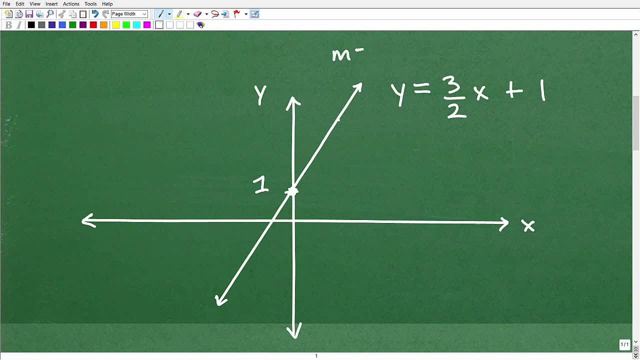 confuse you real. uh, shortly here, all right. so again, slope of this line is three half, so a line that would be perpendicular. again, i'm going to just kind of sketch it, use my sketching skills, maybe something like this: okay, so right here, that's 90 degrees. right now, of course, there's 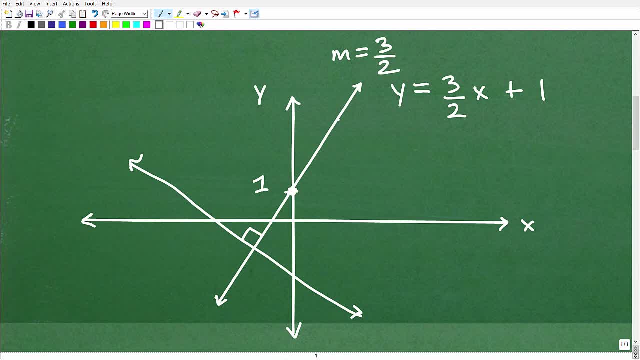 all kinds of lines i can draw. them right here doesn't make a difference. anywhere along this line i can have a perpendicular line. so this line right here has some sort of y equals mx plus b situation going on with it. right, it has an equation that represents this line. 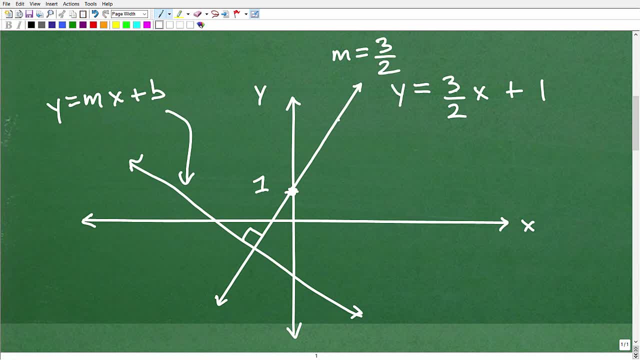 so this line, our original line, has a slope of three halves. okay, what's the relationship, uh, with this slope of a line and a line that is going to be perpendicular to it? okay, so here's the drumroll. right, the drumroll is going to be the negative, reciprocal, all right, so here's what that means. 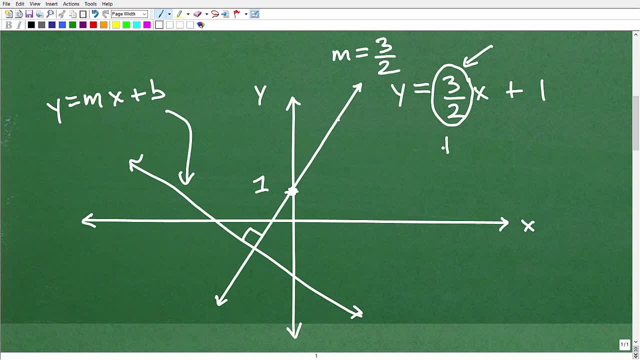 you take your slope right. right here, our slope is three halves. okay, we're going to put a negative sign in front of it and we're going to flip it over. okay, the reciprocal means you're going to flip the fraction over. so that's two thirds. so this line down here has a slope of negative two. 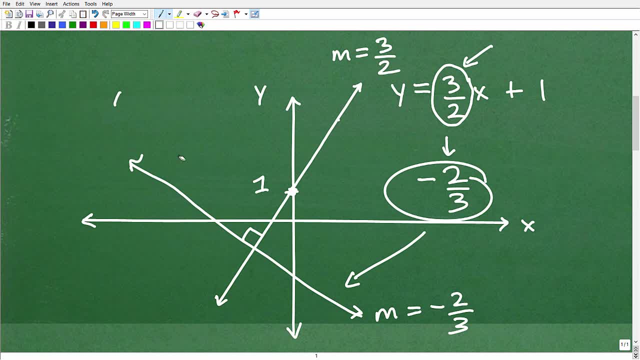 thirds. so let's go ahead and write the mx plus b, and this is the case with all lines that are perpendicular to one another. they have their slopes. are the negative negative reciprocal one another? now, of course they can get a little confusing. we'll do another quick example here. but 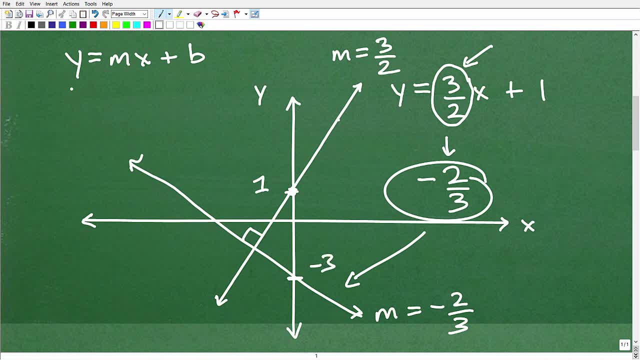 let's say this line is crossing at negative three. so the equation of this line would be: what would be its slope? okay, it's perpendicular to this line, so it would be negative two-thirds x, maybe like minus three. okay, so when you're comparing, is this and this? okay, these two slopes. right now, if i give you negative two-thirds right as my original. 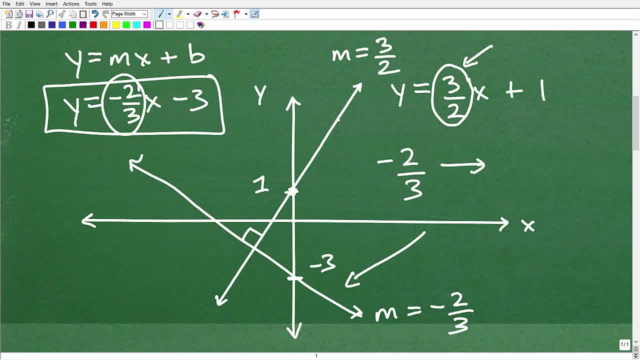 slope. you're like, okay, what? what lines are perpendicular to lines that have a slope of negative two-thirds? well, the the way it works is negative, reciprocal. but really think of it is the opposite sign. okay, so what's the opposite sign? uh, this negative, it's going to be positive. 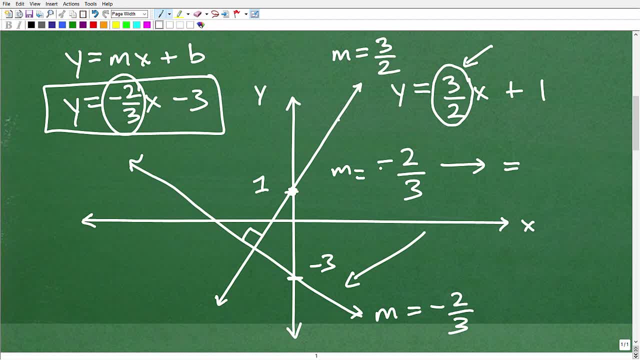 and so we're just going to do the negative of negative three's going to be two line, two-thirds negative, which is positive. it's just the opposite sign. so if i gave you the slope negative, two thirds, the opposite of that's going to be positive. and then you're going to flip this guy so that 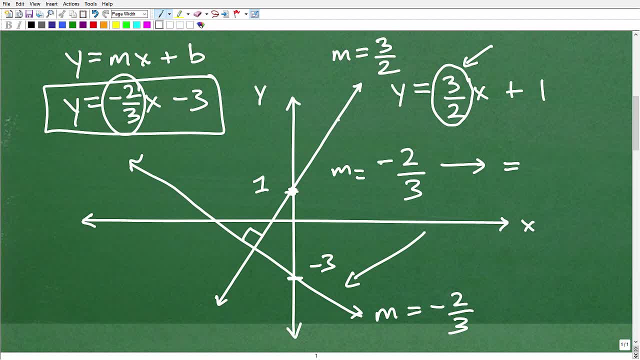 will be positive, right? so i'm going to take the opposite sign: that's positive, and this is two thirds. so i'm going to flip it upside down. that's three halves. of course, we don't really write the positive signs. it's going to be three halves, okay? so there you go. all right, so that's basically it. 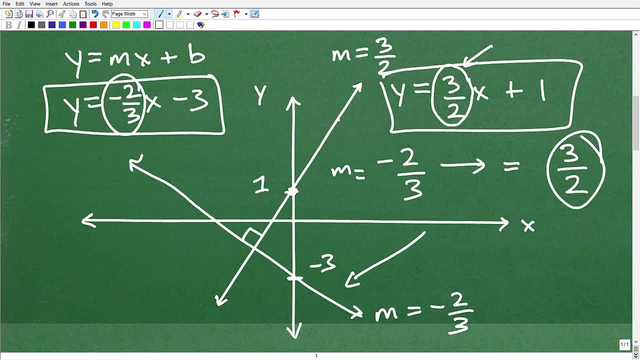 that's the most confusing part generally with students. now again, if you don't understand slope intercept form, or if i give you two points that are on a line you know, for example three, seven and negative one, uh two, and i told you to calculate the slope, then find the equation of a.